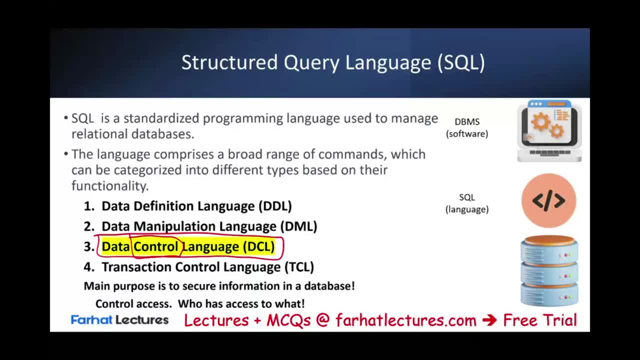 Well, let's think about the purpose of a database. The main purpose of a database is to secure the information, the data in a database and make sure the proper people have access to it. Now, who's going to give us this feature? Well, the control. access is controlled by the data control. 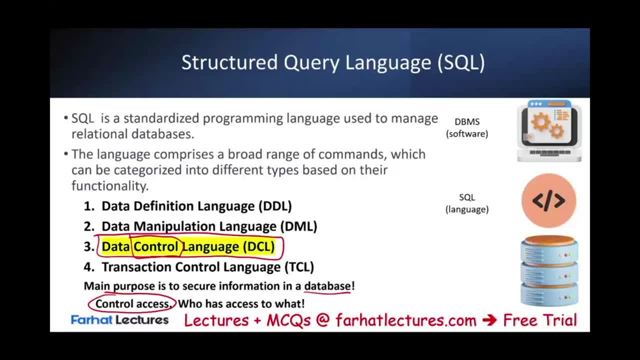 language, and that's why I believe the name of it will tell you a lot. Let's not forget what we are doing. Data control language is an SQL language. What is SQL language? It's a software. It's a language that helps run the database management system. So we would use the software to manage. 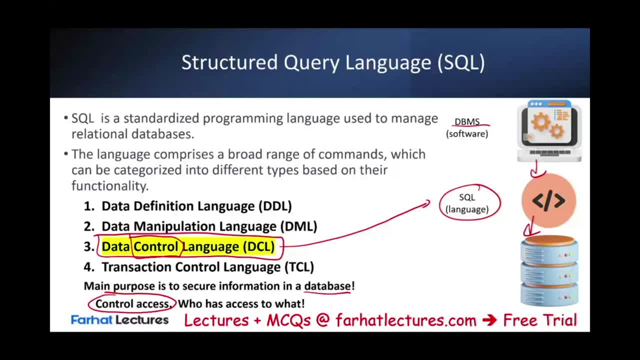 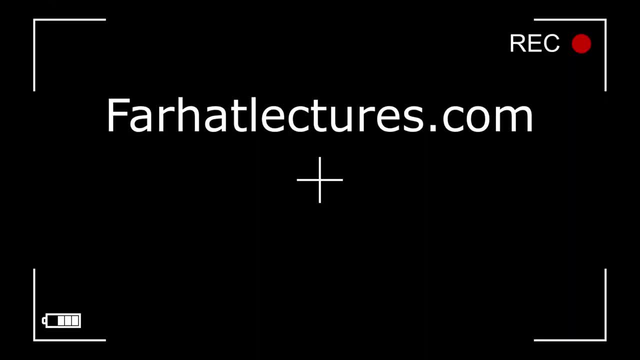 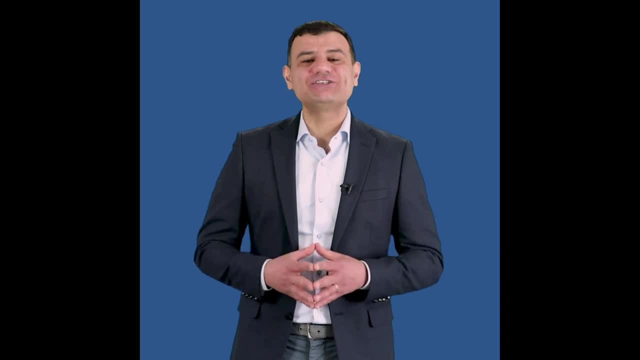 the database. So data control language is part of these languages. Let's go ahead and get started to discuss the data control. Before we proceed any further, I have a public announcement about my company, Farhatlecturescom. Farhat Accounting Lectures is a supplemental educational tool. 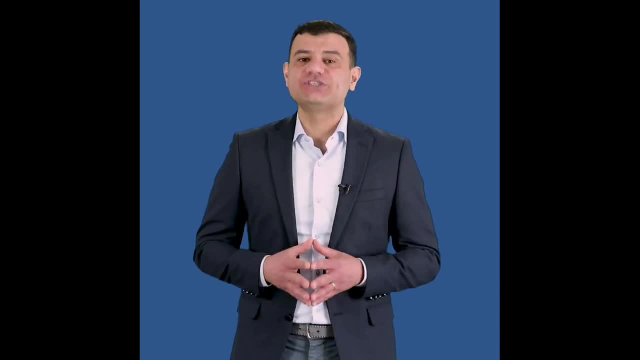 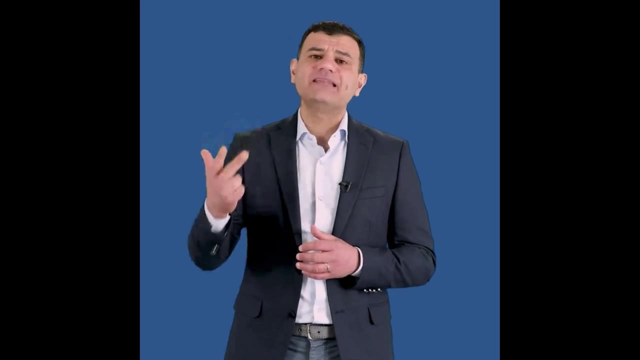 that's going to help you with your CPA exam preparation, as well as your accounting courses. My CPA material is aligned with your CPA review course, such as Becker, Roger, Wiley, Gleam, Miles. My accounting courses are aligned with your accounting courses, broken down by chapter. 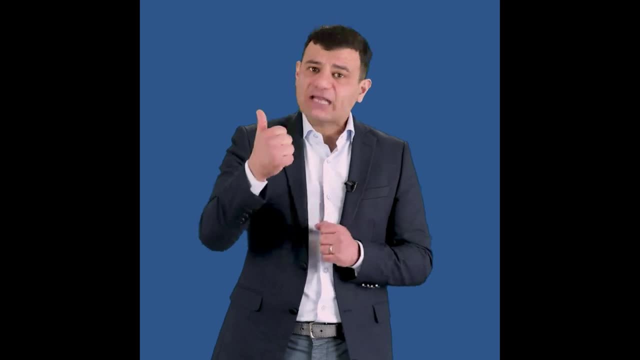 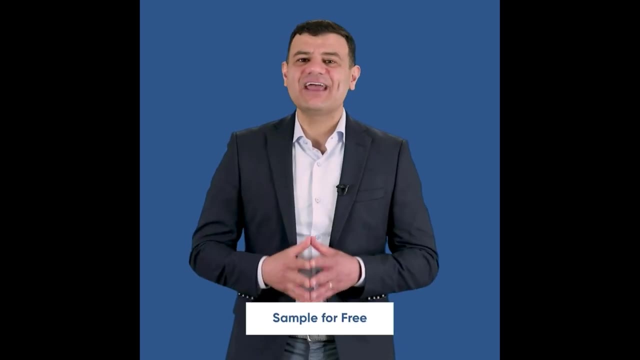 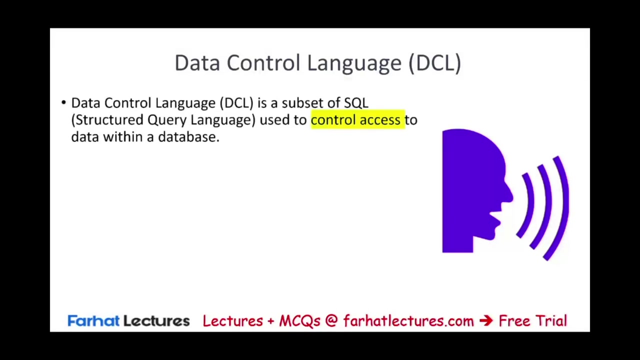 and topics. My resources consist of lectures, multiple-choice questions, true-false questions, as well as exercises. Go ahead, start your free trial today. Data control language. Well, it's a subset of an SQL, the structured query language. 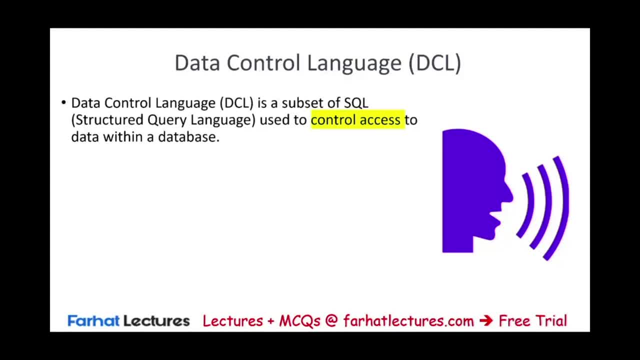 Data control language is a subset of SQL, the structured query language, and used to control access to data, The database within a database, the data within a database. Essentially, DCL commands are used to either grant or revoke access or permission and manipulate data. If I want to give you 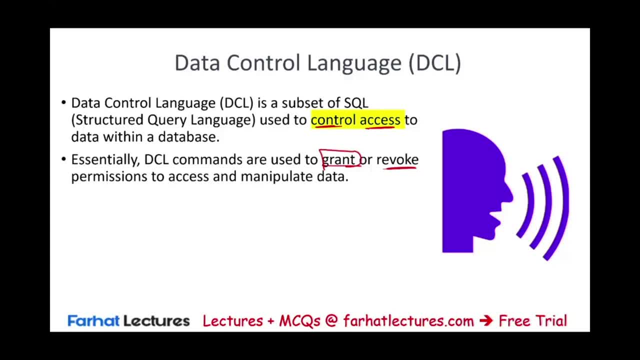 permission, I will give you permission. If I want to take that permission away, I will take that permission. I can give you certain permission to do certain things: update, delete, insert, so on and so forth- And this is crucial for maintaining the security of the database. 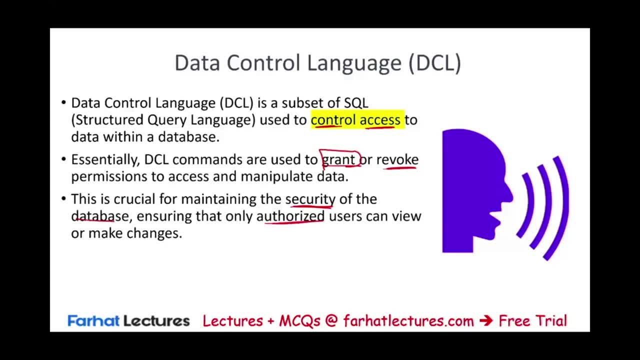 This is making sure that only authorized users can view or make changes as necessary. Now, within this language, within the data control language, we have two commands, usually The grant, that gives access, and the revoke, that suspend or withdraw access. Even the names of those is pretty much self-explanatory. However, within data control language, we 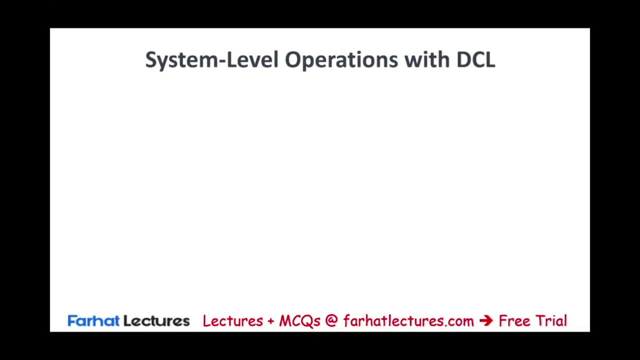 have to be aware of system-level operations and object-level operation. What is a system-level operation? System level, it means the operation here is at a system level concerning the overall database system. This might include the ability to create or drop. Remember, drop is basically delete the database permanently. 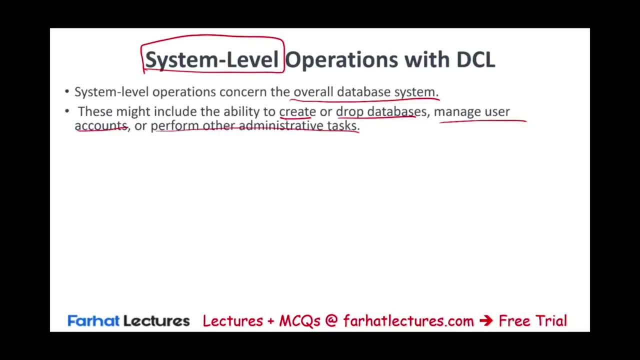 Manage user account or perform other administrative tasks. So these permissions are given at the system level and typically are broader in scope than those at the object level. For example, if I give, I might give you access to the whole database. You can do anything. 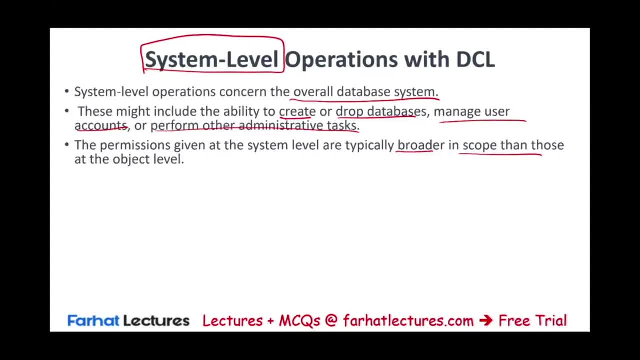 within the database. That's a system level. I'm giving you access to the whole database. For instance, in some databases a DBA might use this command to grant a user the ability to create a new database. So you can create a new database. Here the focus is not on a specific database object. You are not given. 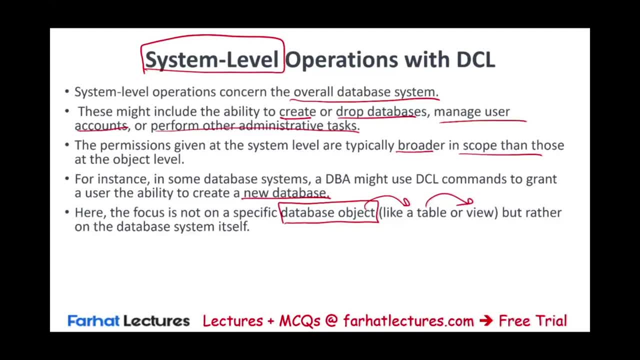 access to a specific table or a specific view, but to the database overall. For example, in some SQL system you might provide the user the ability to create a database with a command like this: grant create database to whoever the user to the user This way. 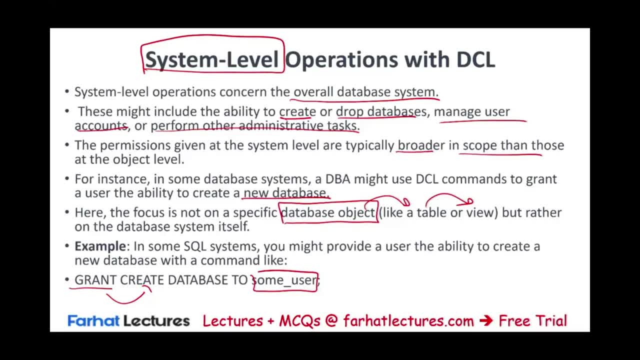 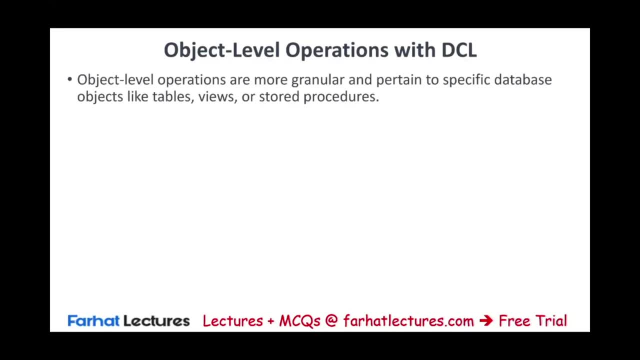 the user will have the ability to create a database. Then we have the object level operation, which is within the data control language. Those are more specific, granular. They pertain to specific database object like tables, views or stored procedures. Now, when you are granting, 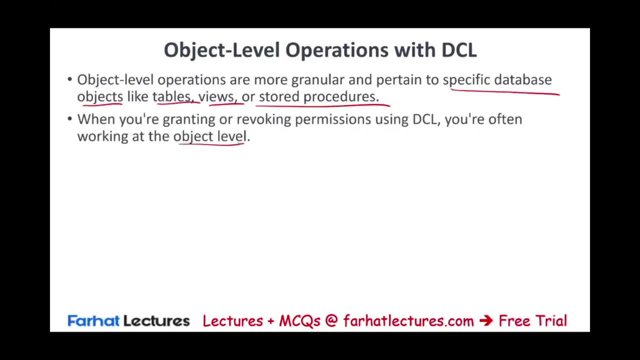 or revoking permission. Here you are often working at the object level. here This is usually for lower staff, you would assume The common operation that can be controlled at the object level would include select, which is only read data, retrieve data insert, add new data, update, modifying. 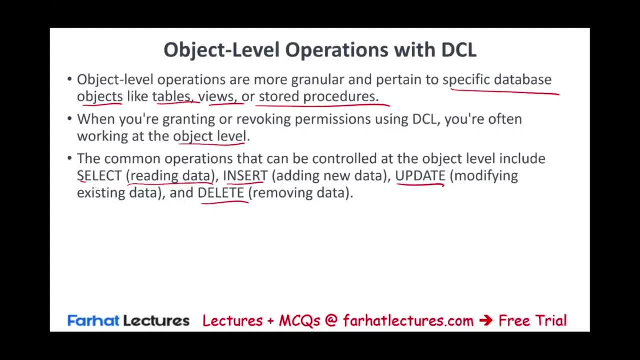 existing data or delete, removing specific data. Here you are giving access to a specific task. DCL command here can precisely control which users or role have permission on which object. An example will be to allow the user to read and modify data in a specific table. You might. 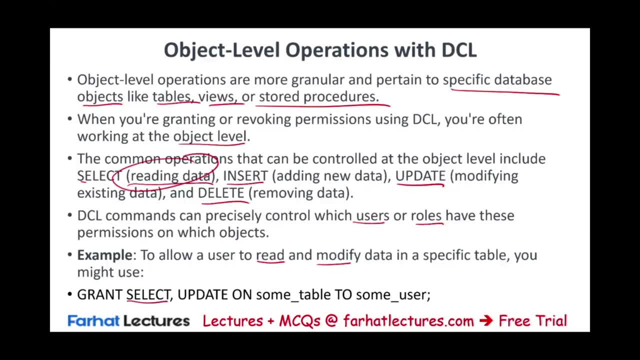 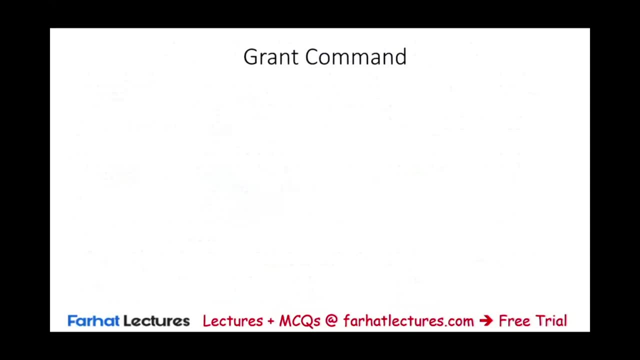 use, grant, select What is select, Read data, update on some table to some user And this is what you are granting to view and update, whatever the table is and whoever that user is. Let's take a look specifically for the grant commander Just to kind of see how the 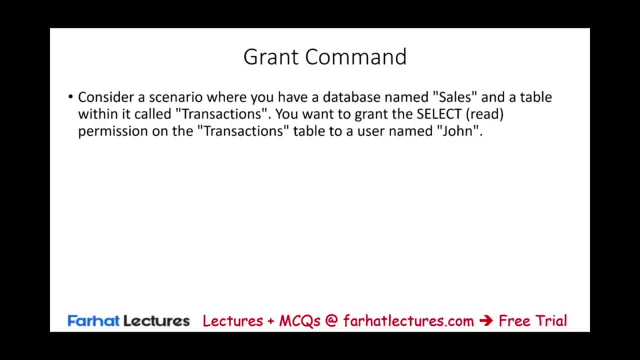 grant and the revoke command are, they are used. So consider a scenario where you have a database named sales and a table within that database called transaction. So remember, the whole database is called sales and we have a table and that table is the transaction. 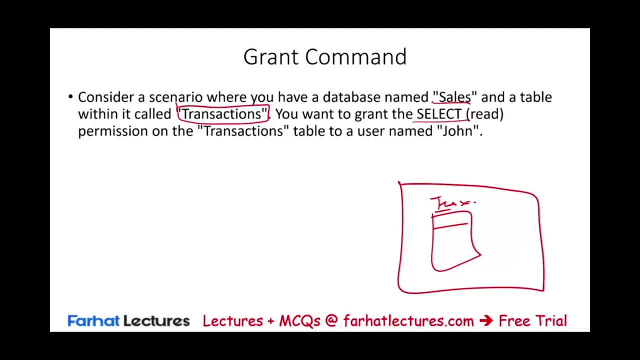 table. You want to grant the select, which is the read permission, to a user named John. So user the grant command. you can say grant select on sales transaction to John. This will allow John to query and read. You can read the data from the transaction table, but John cannot modify Later. if you 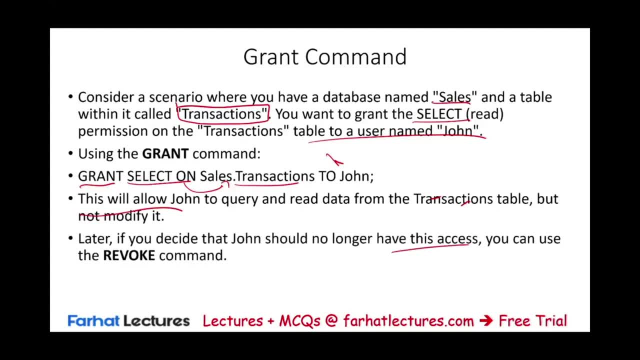 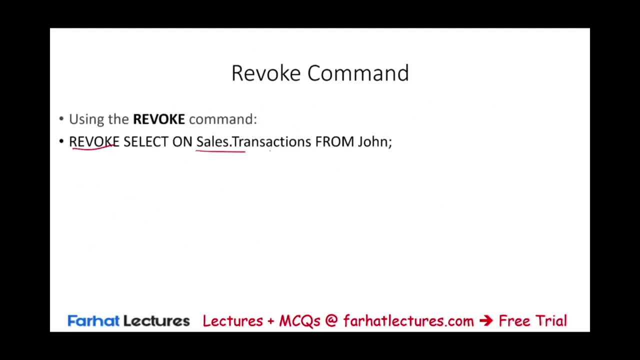 decide that John no longer should have access. well, you can revoke this command. How do you revoke the command? Using the revoke command, you would revoke select on sales transaction from John and this will remove John to be able to query the transaction table. 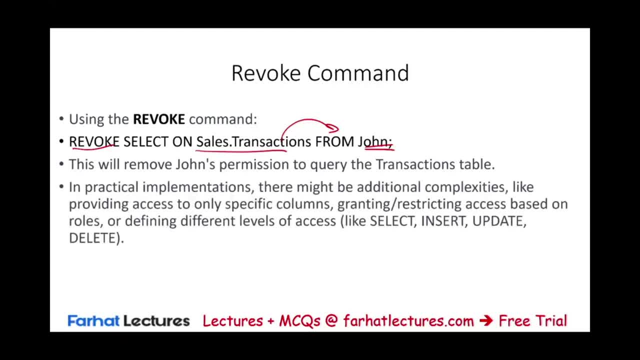 Now in practical- just kind of practical implementation, there will be additional complexity. So you might be looking at providing access to only specific column, granting or restricting access based on roles or defining different level of access. In the real world this looks. 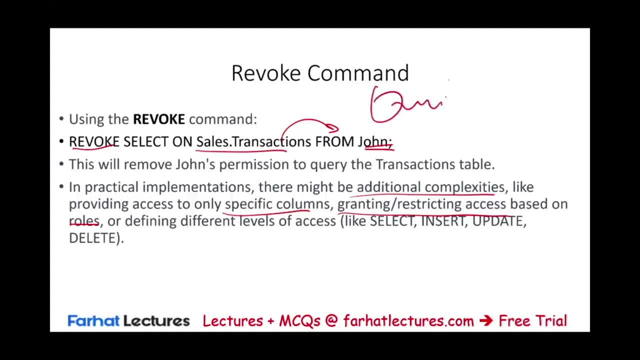 it might be a little bit different. For example, I teach a course called QuickBooks and within QuickBooks, if you create the company, you could give access to users, And this is basically a form of data control language. Okay, but the above example should give you a basic. 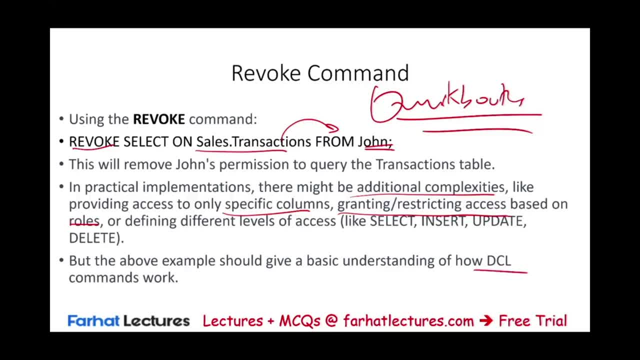 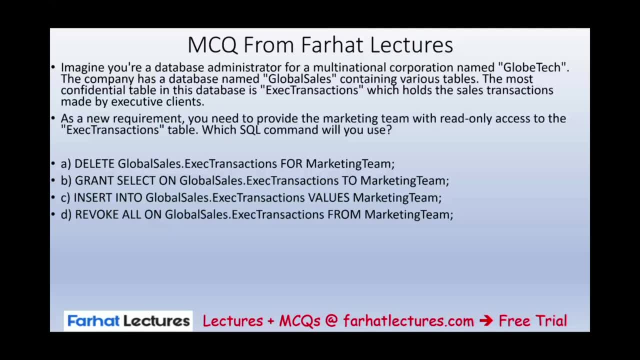 understanding how DCL- how DCL works- commands work. Let's take a look at this multiple choice question from Farhat lectures. that's gonna help you understand or consolidate what we just learned. Imagine you are a database administrator for a multinational company, Globetac. the company has a database named global sales containing 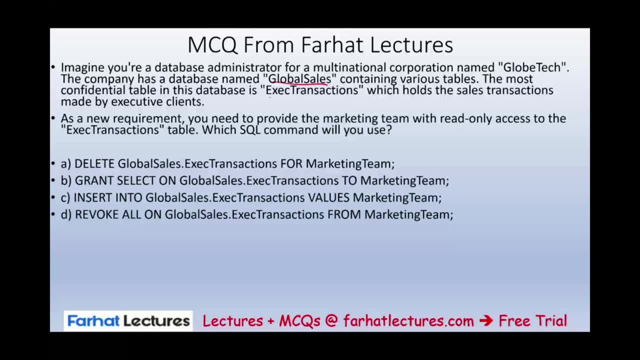 various tables. The most confidential table in this, in this database, is executive transaction, which hold sales transaction made by executive clients. As a new requirement, you need to provide the marketing team with read-only access to the executive transaction table. Which SQL you would use Well, would you delete? 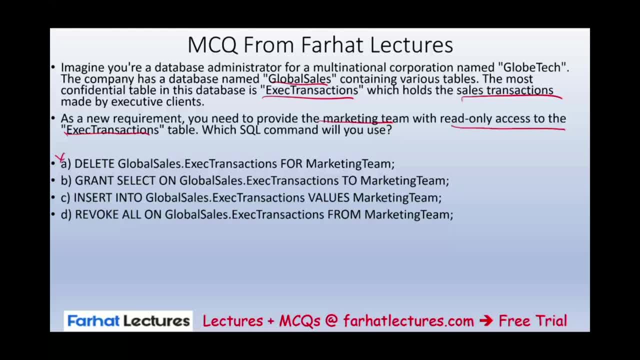 Would you delete? And the answer is no, You would not delete. You're not deleting anything. You're not deleting anything, Would you? you're not deleting any record here. Would you grant select? That's why I think that's what you're. 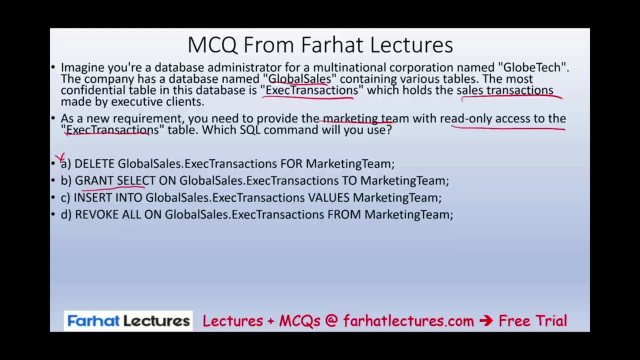 trying to do? You're trying to grant them the ability to view, So grant, select on. this is the global sales. is the database dot the table. executive to the marketing team. I believe B is a good answer. Insert new global sales values, marketing teams. This is to add a record. We're not adding any record. Definitely we're not. 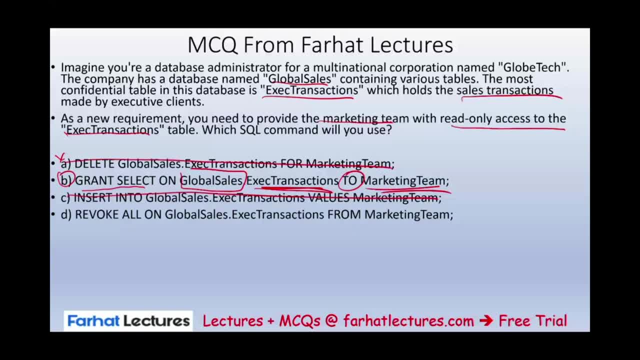 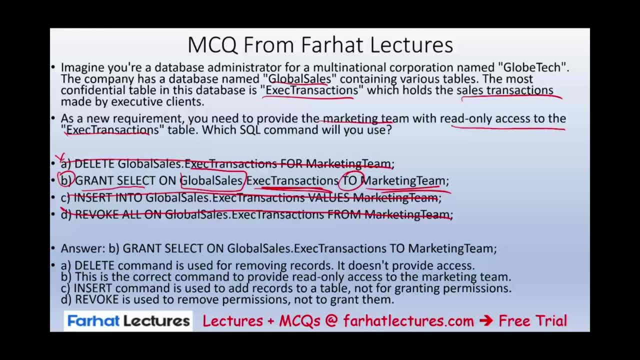 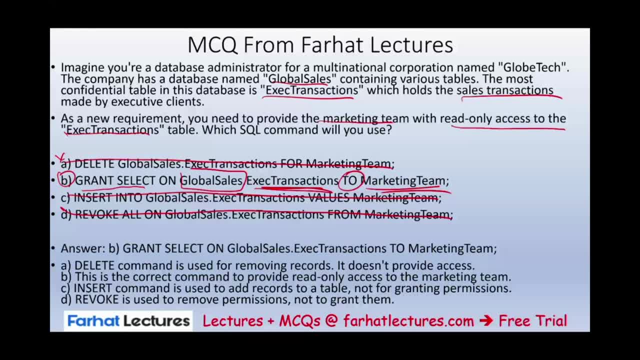 the table. dot the name of the database. dot the name of the table to whoever you wanted it to give it to, which is the marketing team. What should you do now? Go to Farhat lectures. Look at additional MCQs. That's gonna help you. 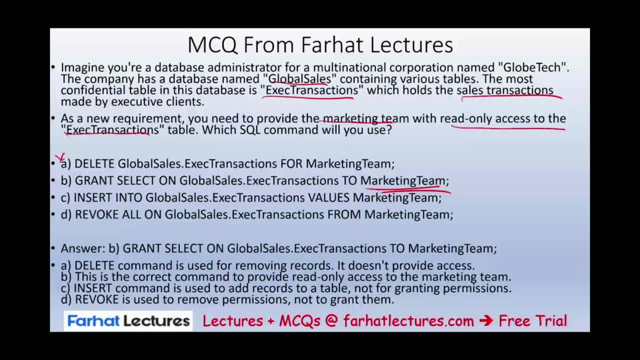 understand data control language Just like an SQL language. You want to be familiar with this for your CPA exam- accounting information system As well as any other professional certification. Invest in yourself, Good luck, Study hard and stay safe.